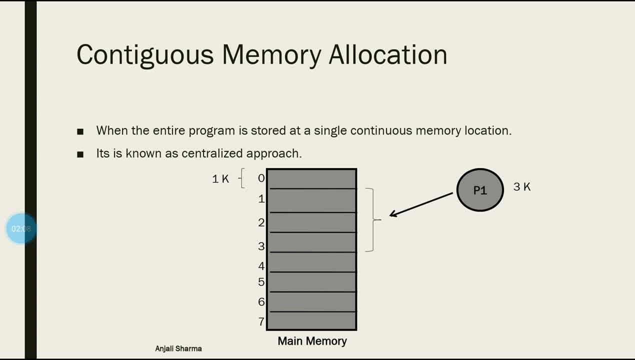 size. that means there should be no gap between the blocks that acquire process p1. that is, continuously the blocks will be acquired therefore from location 1 to 3 contiguously will be allocated to process p1. that is the contiguous memory allocation right in contiguous memory allocation. 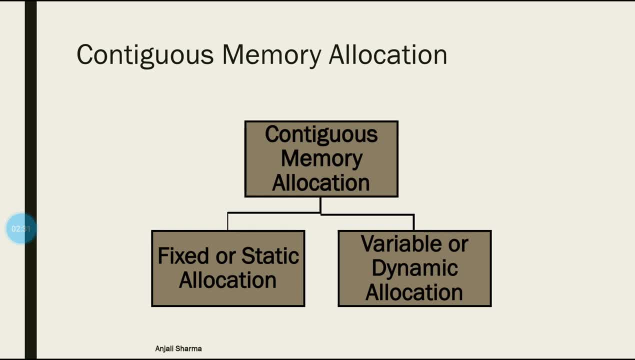 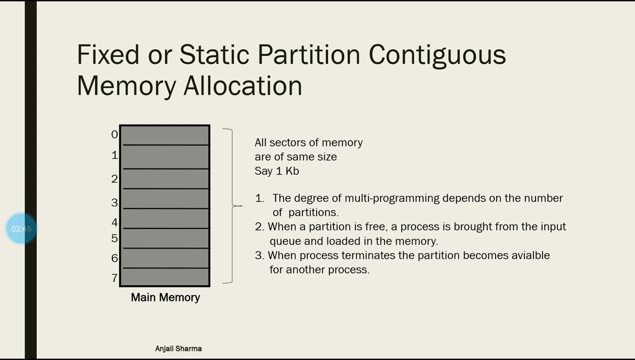 can be divided into two types: one that is the static or the fixed allocation, and the other is the variable or the dynamic allocation. so let us see them individually: fixed or static? dynamic allocation is that that all the sectors of the memory will be of same size. that is partition. 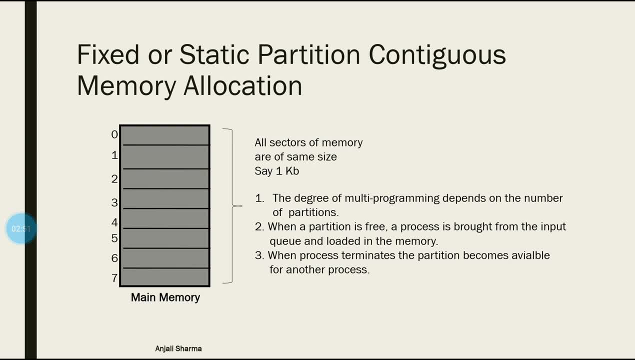 zero will also be of 1k b, partition one will also be of 1 k b and all other partition, that is, the total partition, will be of same size. the degree of multi-programming depends upon the number of partitions, obviously that many partitions will be holding up the processes. therefore the degree of 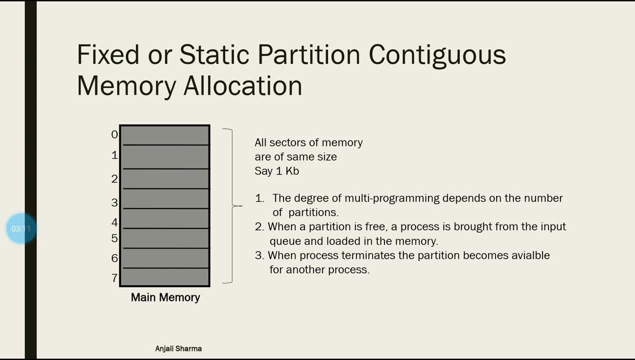 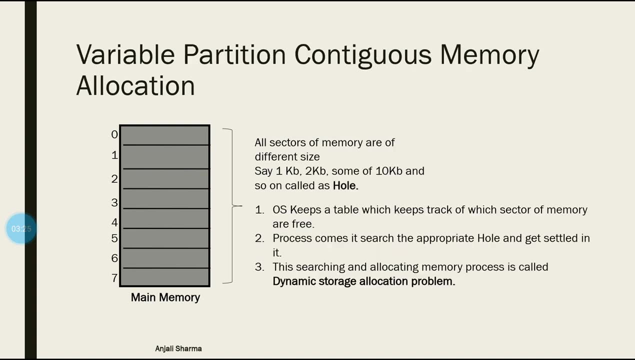 multi-programming depends upon the number of sectors that we have in the main memory. when partition is free, a process is brought from the input queue and loaded in the memory, and when the process terminates, the partition becomes available for the other processes. the next type of partition is the variable partition, in which the sectors are of different. 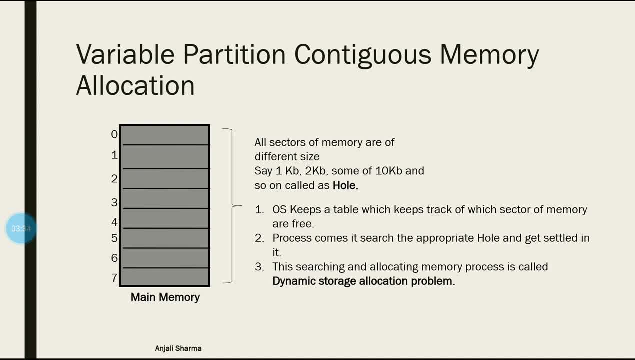 sizes. for example, one sector will be of 1 kb, second will be of 2 kb and others will be of 10 kb or 20 kbs, and so on. that is, there is not uniform partitioning between the sectors. so that is the variable contiguous memory. 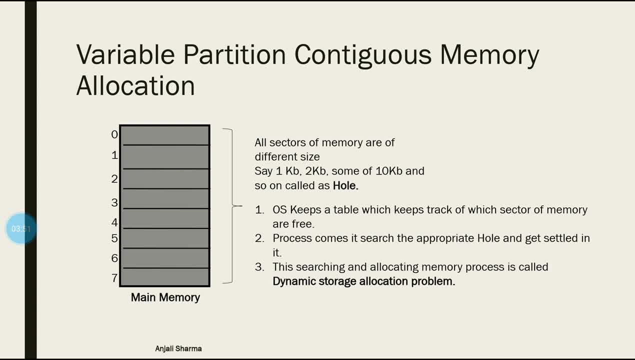 allocation, but here also the processes which will be coming will be occupying the memory locations or the partition in a continuous manner. now the operating system have to keep a table which tracks the number of sectors in the memory that are free at a time. the processes comes and search the 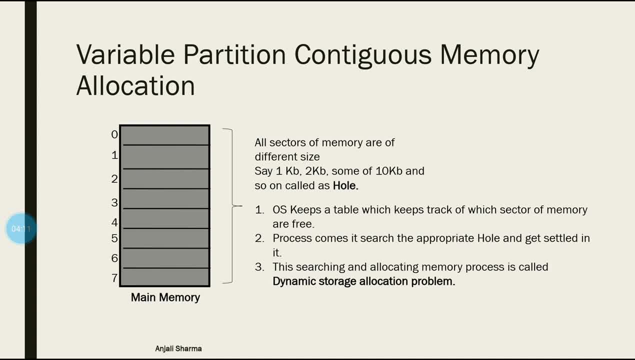 appropriate hole or a free memory location and get settled in it. this searching and allocating memory processes is known as a dynamic storage allocation problem. that is the process have to come and find out a particular position to settle down without having much loss of memory. so that is.